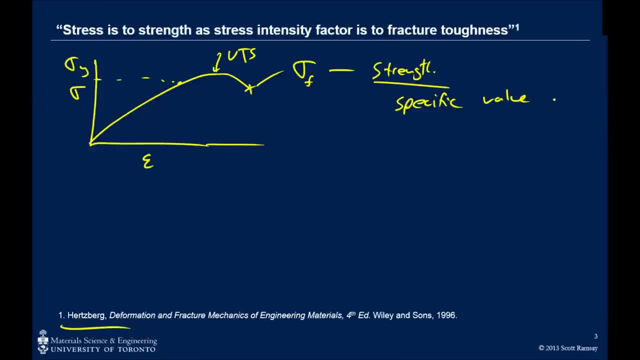 Okay, Specific value Of stress. So now we have the stress intensity factor K And a specific value of that is the critical stress intensity factor. That is the stress intensity factor when the crack becomes critical. The crack has grown to a sufficient length that it is critical. 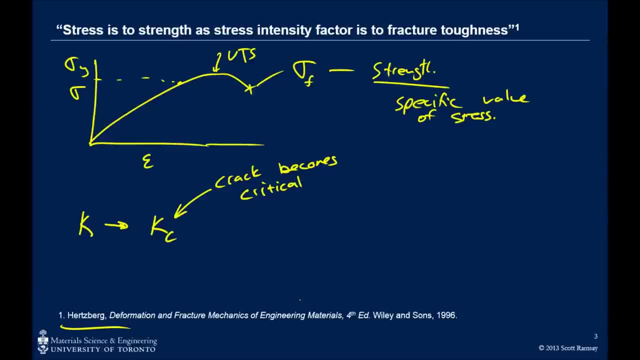 That is, The propagation is now going to become unstable. And more specifically, actually we're going to look at the most common form of the stress intensity factor, Sorry, of the critical stress intensity factor, The plane strain fracture toughness K1C. 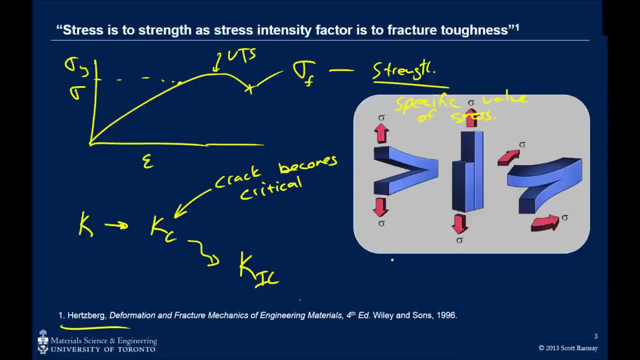 Okay, And the one, the Roman numeral one there, actually refers to mode one, crack displacement, That's crack opening. Just out of interest to say here: crack two, mode two is sliding And mode three is referred to as crack opening And mode three is referred to as tearing. 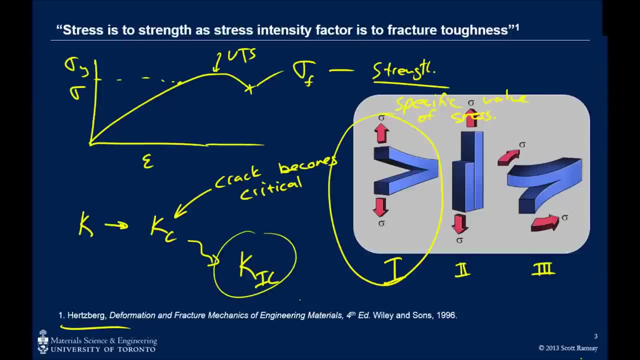 But mode one is what we're going to be interested in. That's the most common form of crack displacement that we'll encounter, And so the K1C is the fracture toughness, And remember that the fracture toughness is a specific value of stress intensity factor. 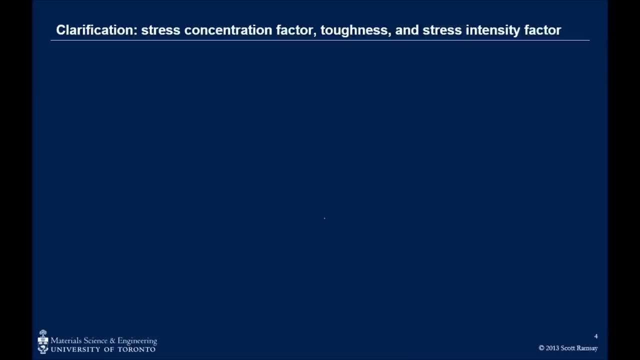 So the last thing I'd like to just address is this: clarification. We've covered a number of things here, Okay, Okay. Okay Okay. Stress concentration factor, which was covered in the synopsis number one, you'll remember, was K sub T. 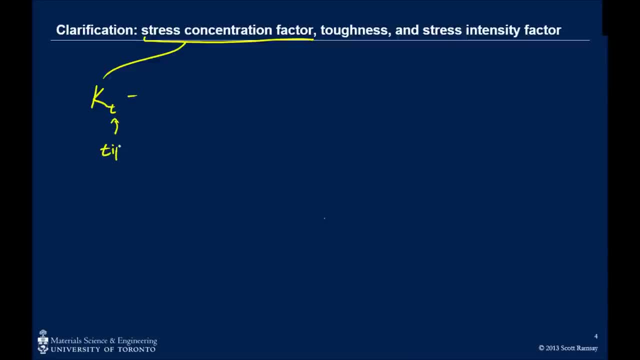 And that's the stress concentration factor at the crack tip. And that was just the ratio of the maximum stress at the tip of an elliptical crack in our case to the applied stress. Okay, So stress concentration factor, how much is the stress concentrated? 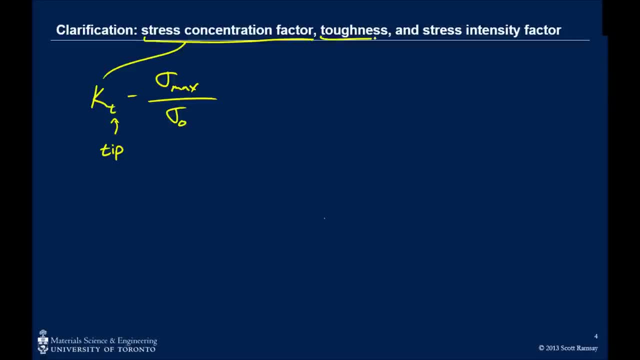 And now we've also- We've earlier in the year- seen this property of the toughness, and we define the toughness as the area under the stress-strain curve up to fracture. Okay, So that's the toughness. That's essentially how much energy is involved in breaking and fracturing the sample.